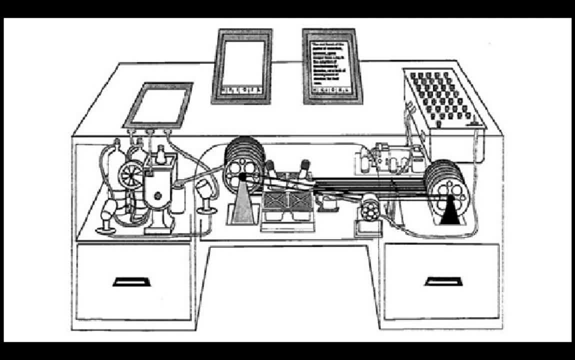 The Second Time. So he wrote a couple of comments in the- As We May Think- article in the Atlantic Monthly, which originally, in fact, was written in 1939, wasn't published until 1945.. A lot of the things that he talked about in fact led towards what would be the World Wide Web or hypertext. 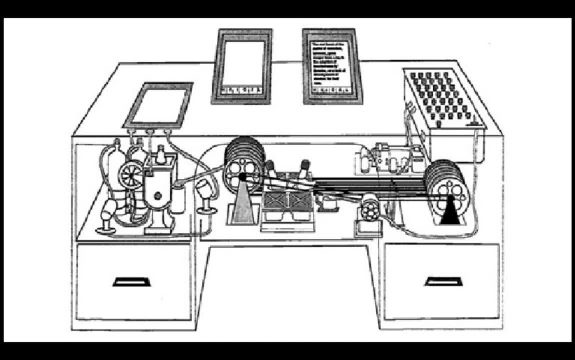 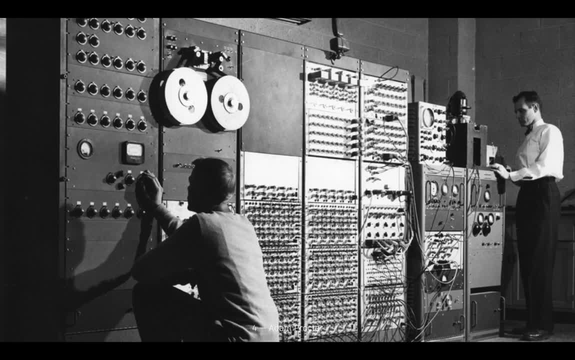 and that was back in 1945.. Now, at this time, obviously, computers were not small. They certainly weren't personal computers. They would often take up huge rooms and spaces. But in the In 1960, a guy called JCR Licklider wrote a seminal piece called Man-Computer Symbiosis, in which he felt that in not too many years human brains and computer machines would be coupled together very tightly and that the resulting partnership will think of as no human brain has ever thought before and process data in a way that has not been processed before. 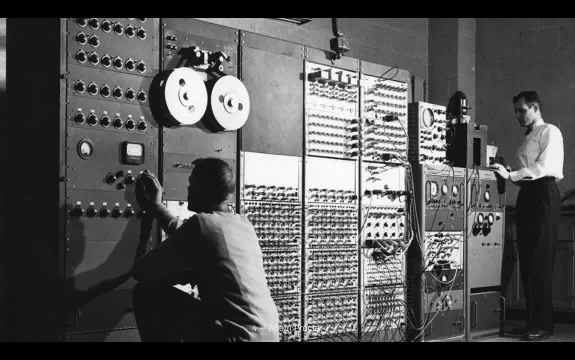 So that was in 1960.. Obviously, one of his immediate goals there was the fact that these computers were huge and that people had to share those resources, and so ways of being able to share and time share computing was important, and this idea of having some sort of input and output display for communicating information in real time was something that he considered. 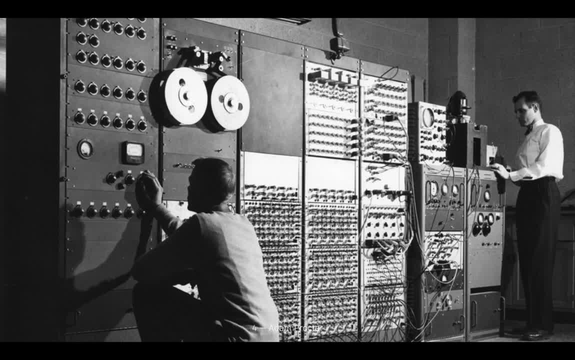 And so he really felt that man and computer would be able to come together pretty rapidly. It didn't quite happen. It didn't happen as fast as he felt, but these days, of course, when we use the iPhone and various other things, they are augmenting our thinking, and so this is something to consider, and a lot of these people here were looking at ways that we might extend our thinking through human-computer interaction and really a symbiosis of those two opportunities. 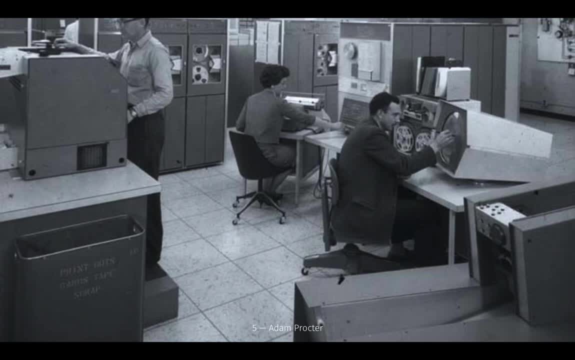 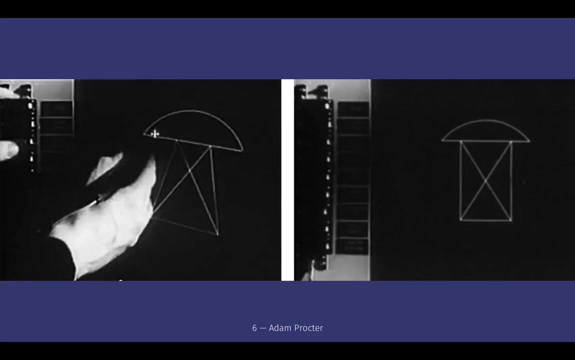 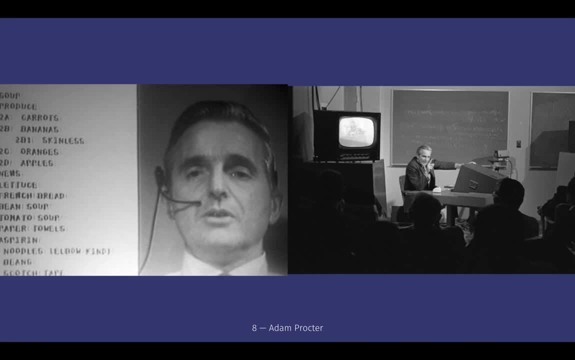 This demo, which is well worth watching in detail, really introduced a whole host of features that we know today. It was at this point that the mouse was first shown here we had. he goes and creates a shopping list where he can delete, remove and move items around. 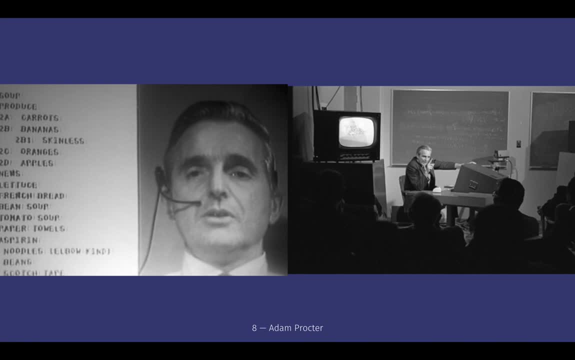 He does a number of things that really are- now, you know, standard on every computer that we use, So this is definitely something to look at. it's quite a long demo, but you'll get the idea. and again at the beginning, 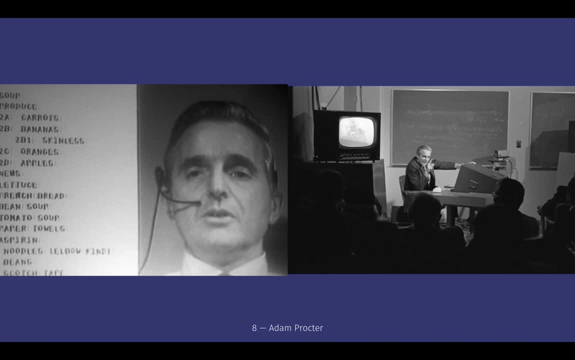 And this is the demo which is well worth seeing in detail- really introduced a whole host of features that we know today. the demo: he talks about the ability to have a computer that was always on and would work at the instance of reactions to you, and this was in 1968 and many. 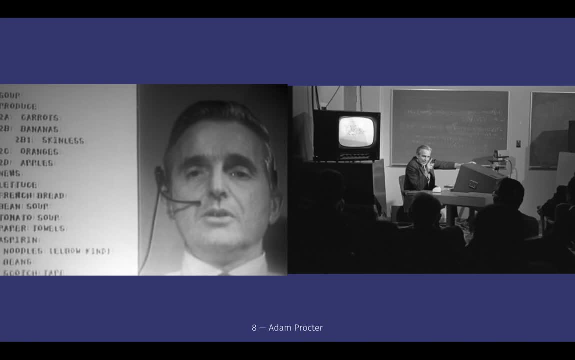 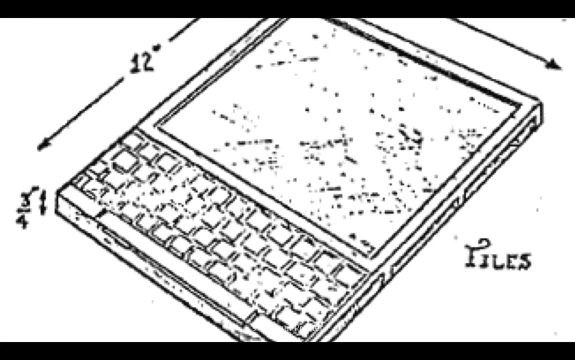 argue that a lot of Doug's thoughts and things here are still to be realized up until this day and some of the systems that he had were, you know, way ahead of its time. in 1972, you know, in again inspired by, you know, Engelbert and 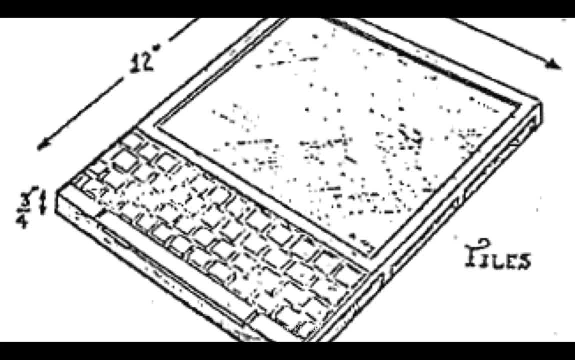 others. Alan Kay wanted to create something called the diner book, and this is actually a sketch of his concept, and he was looking actually in in learning theories from Bruner and puppet around how we might use a digital tool for learning, and so he created what's called the diner book and this you know. 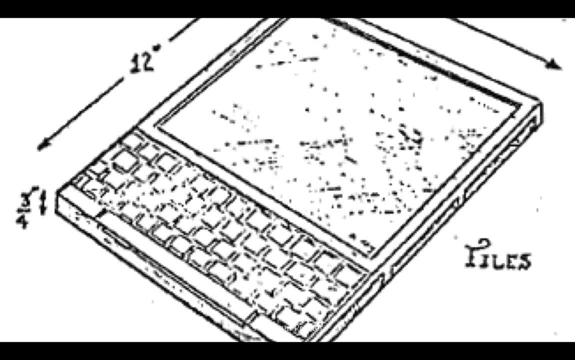 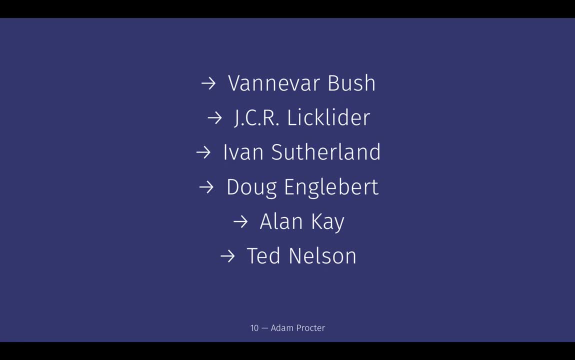 obviously looks very much like, you know, a laptop or an iPad with a screen connected at the bottom. and this is in 1972 and he called it a personal computer for children of all ages, the diner book. and so we see here these kind of key people: Bush, Licklider, Sutherland, Engelbert and Kay- really, 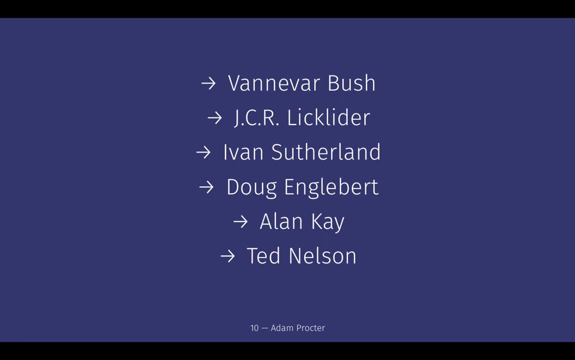 inspired at this point by each other to push forward what would become personal computing. Ted Nelson- there is another character to investigate and look up. so Ted Nelson invented terms, hypertext and hypermedia and is a forerunner to what would become the World Wide Web. but 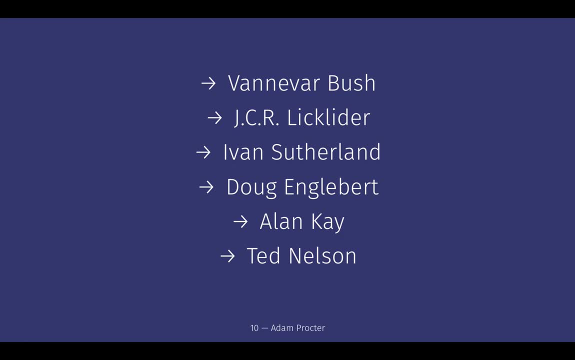 had some very different approaches to that and in fact, again, a lot of people are looking at his work now and reinvestigating it. with the level of computing, we have to see whether there might be alternative interfaces there. so Ted Nelson, another person to relook up, and the Xanadu project, which is 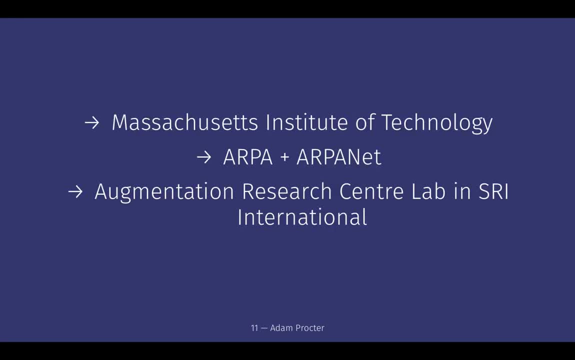 spelled with an X. some other areas of interest connected to this is obviously the massachusetts Institute of Technology, Arpa, and of course the Arpa Net, which would be the forerunner for the internet, and we've mentioned there. the augmentation research center lab is another place to look. so this was all. 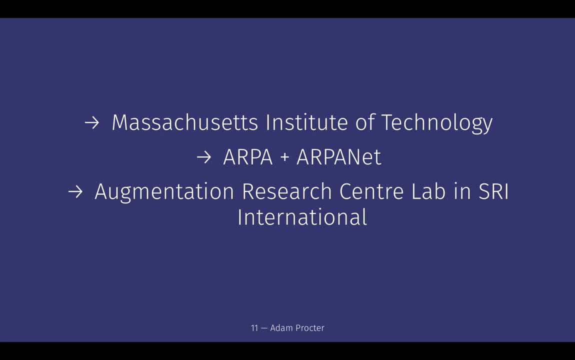 happening in the sort of you know nineteen, fifties and nineteen sixties where we were starting to see this idea of how computers and humans might interact together. we had some very crude graphical user interfaces and of course, Doug Engelbert's- chopper of all demos- really did showcase that ability to not use programming but have a visual interface. 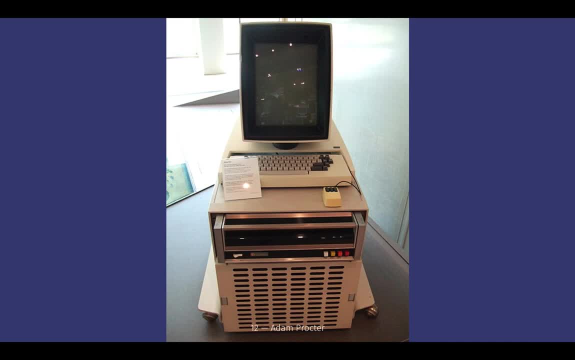 that will allow you to interact with the computer. this is a xerox auto. it was the first computer designed from the inception to support a graphical user interface, which would later become, obviously, desktop metaphor. the cpu for this actually resided in in the entire cabinet underneath, so 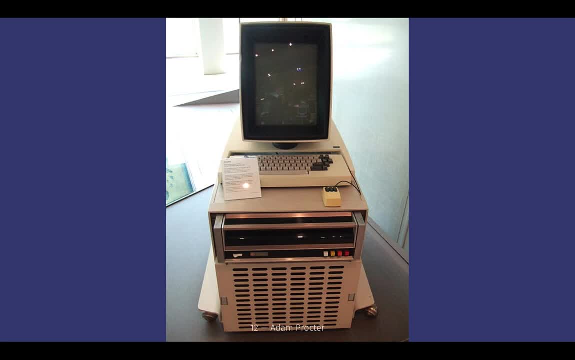 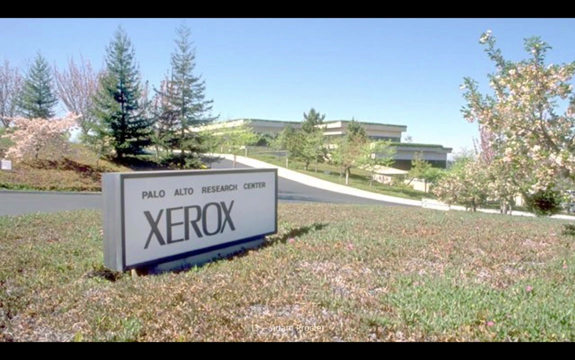 a lot smaller than the computers. uh, you know, prior to that, and this is in like 1973.. so this is about a decade prior to actually mass market getting these graphical user interfaces, and they built with the custom chip that would fit into that cabinet. so xerox park is the place where 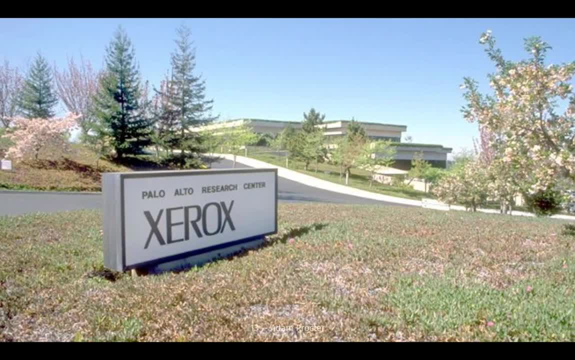 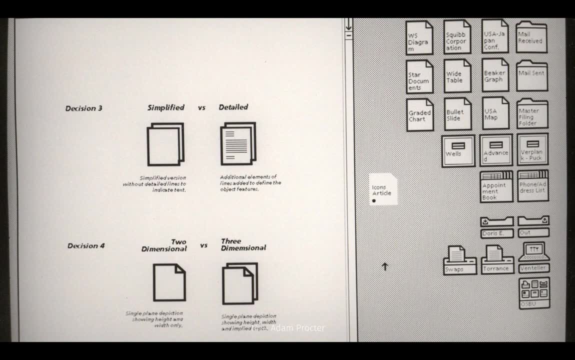 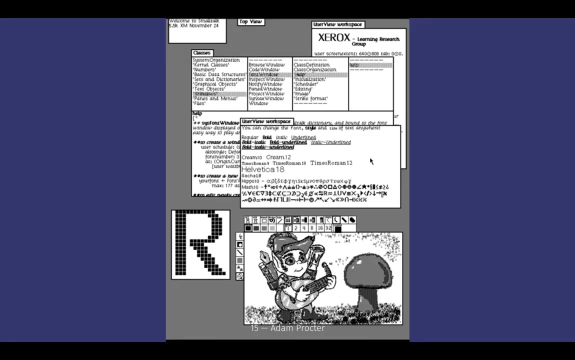 the modern graphical user interface started and it was started with the xerox operating system which we can see here and you can see something. obviously, some key things are very much like what we see today. this is actually an implementation of an operating system built on small talk which alan k used for the dyna book as 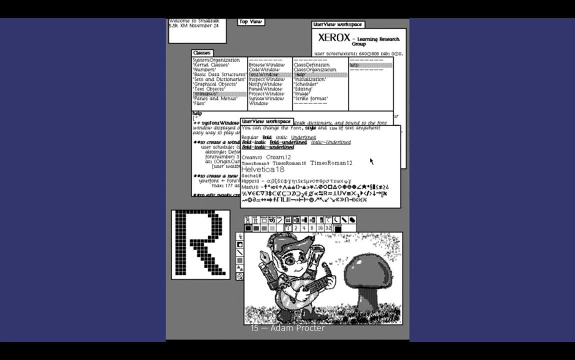 well. so this again is again through xerox and this is looking at the learning group and small talk was also, you know, seen as an exemplifier of this human computer symbiosis. so we see those clink, those links through right now from the 1960s into 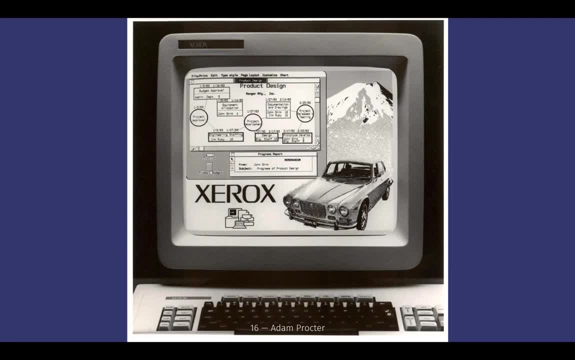 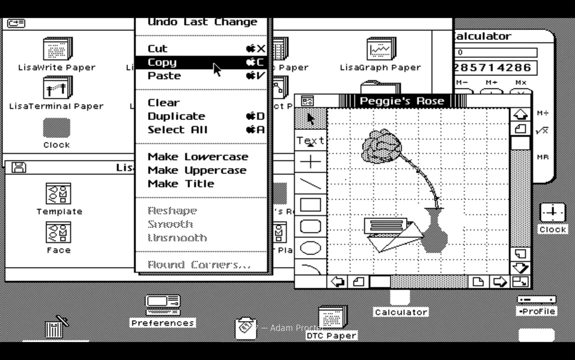 the 1970s. this is the xerox system, and what's key to understand here is that in 1979, apple, under the sort of you know enthusiasm of jeff ruskin, steve jobs visited xerox and they took a long look at what was the xerox operating system and also what would be xerox star. so this is. 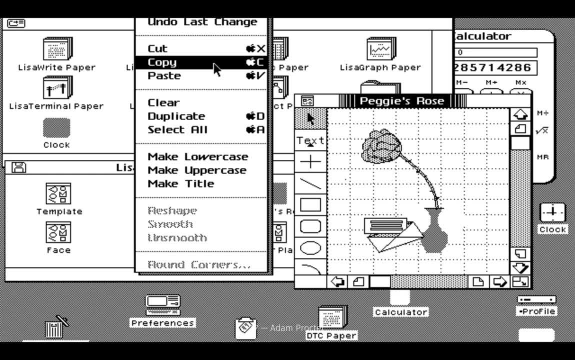 the xerox operating system. as you can see, the xerox operating system was a fairly exciting project to have to face many of the politicalogo's of the past, because it was in 1983 and a lot of the metaphors and things that we see from the xerox system were quite clearly inspired. 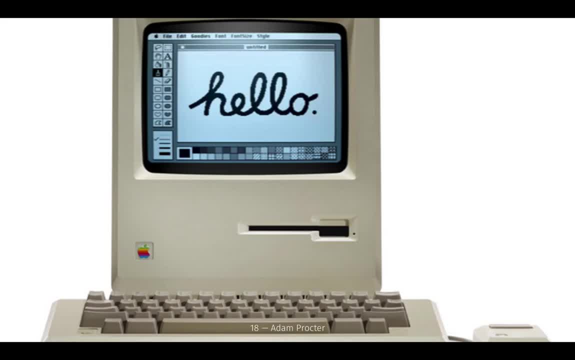 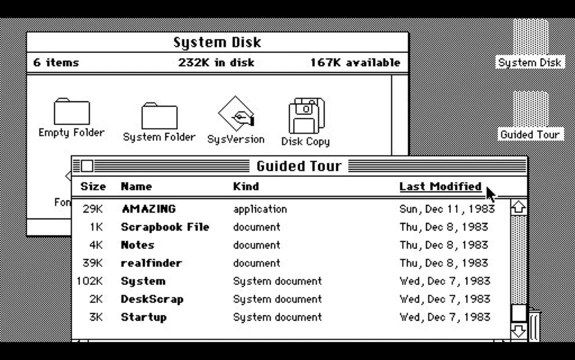 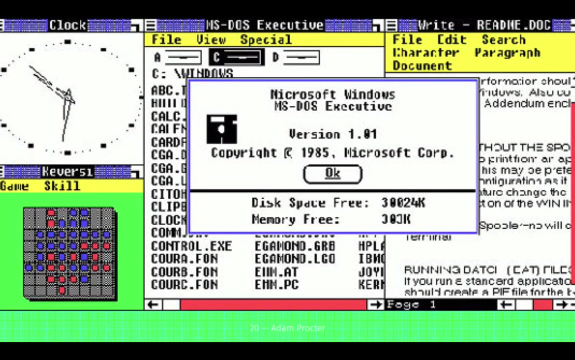 and, provided you know ways, for apple to release the lisa in 1983. so this is probably one of the first sort of personal computers that is now becoming mass market. it was in 1984 that apple- so that's menus, files, folders, these kind of things- really all born from xerox park. it's in 1985 the 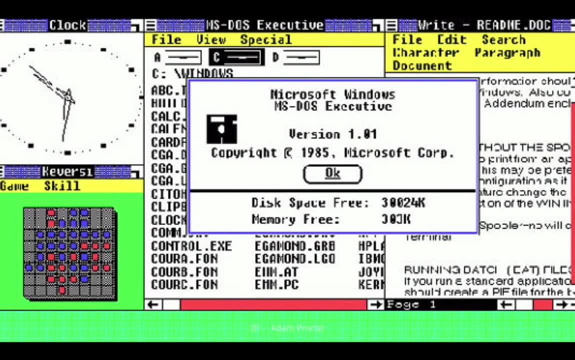 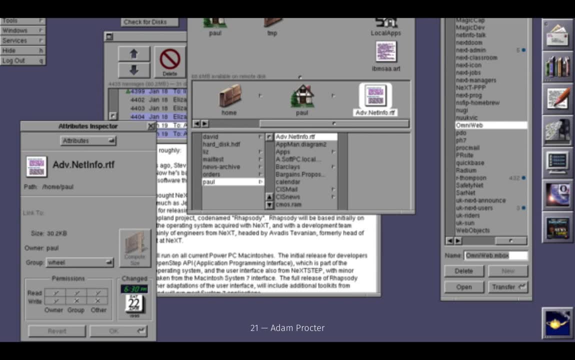 first version of Windows is released and again trying to borrow a very similar, you know, interface style, looking particularly this point more towards for the Macintosh. and in 1988, next step, which is the operating system that Steve Jobs when he left Apple after their issues around, in fact the 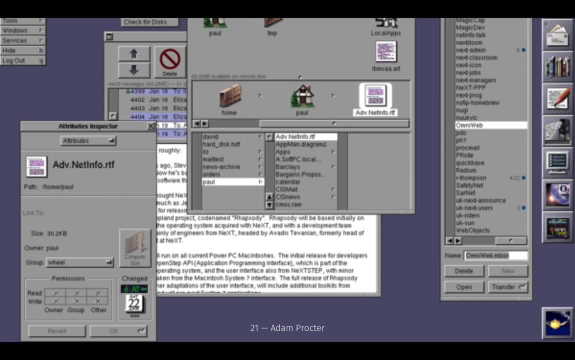 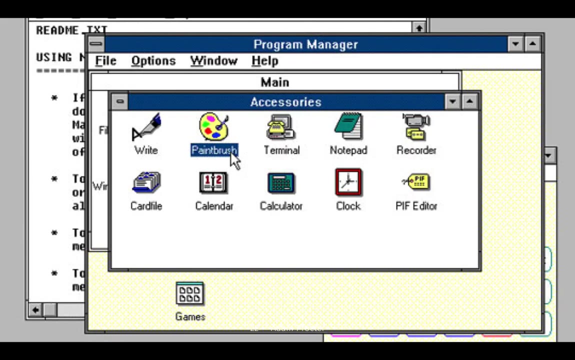 Macintosh and other systems. he went on to form a company that built next step, which was a new operating system, and in fact this was a system in the world wide web would be invented on the web. But here you can see- obviously you know some of the more icons. again, a very similar interface. 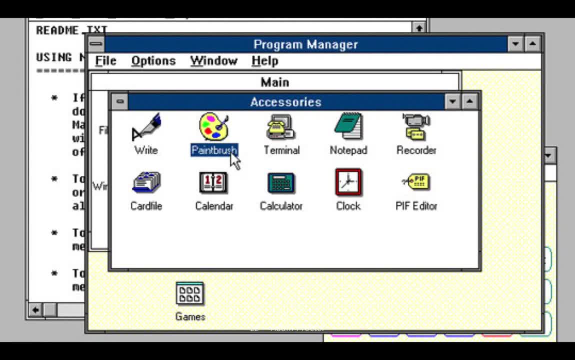 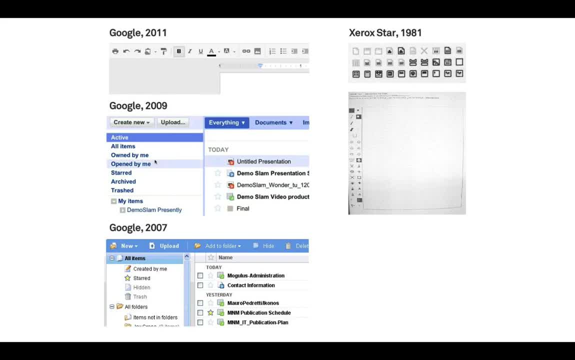 Windows 3, released in 1990, again utilizing the same thing. at this point we're starting to get much more color involved. in fact, if you look at, you know, today's interfaces, we see, you know Google, the Google Office suite. here, really, you know utilizing and taking advantage of what would be. 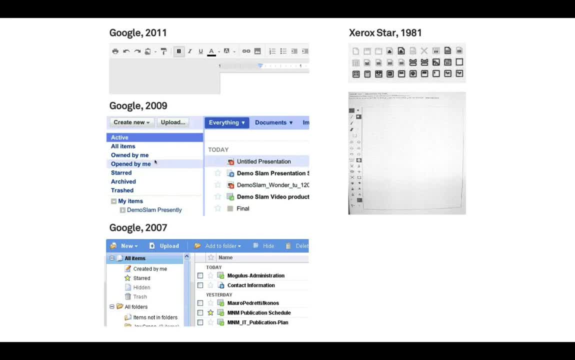 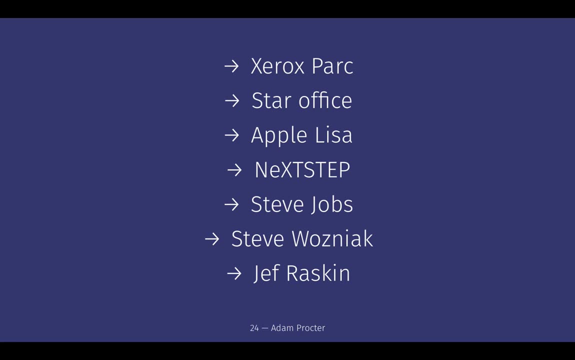 the implementation of Xerox stars own. so icons, graphical user interface- not many things really have changed in that instance of in the computer have become much more powerful. so few things, just to bear in mind. Think about it so, and this is kind of a way to understand it is Xerox Park particularly Star. 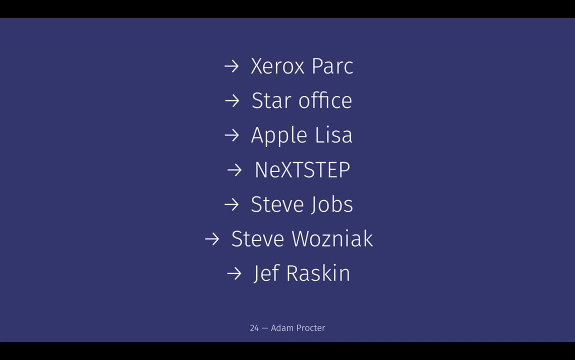 office know those interfaces really inspired the systems that went on to be the Apple Lisa and, of course, the Macintosh. Next step took that to another level with steve jobs, steve wozniak and jeff ruskin, also key players in the hardware. 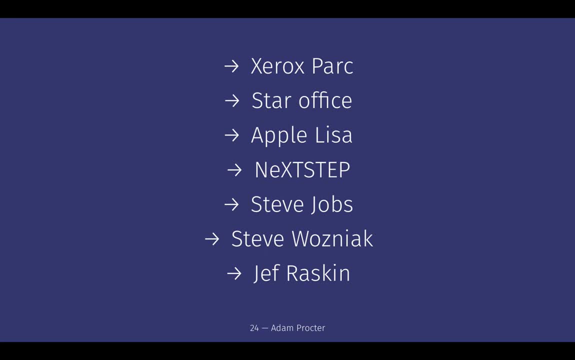 and the implementation of these os's. often steve jobs is credited with these things, but of course you know it wasn't without others that he did the things that he did. of course we see the operating systems today evolve slightly and windows- obviously 8 and windows 10- is starting to push this kind of. 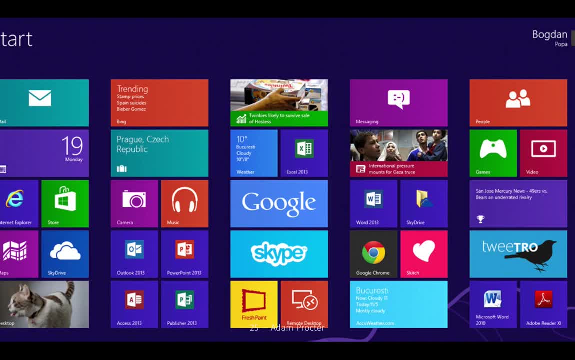 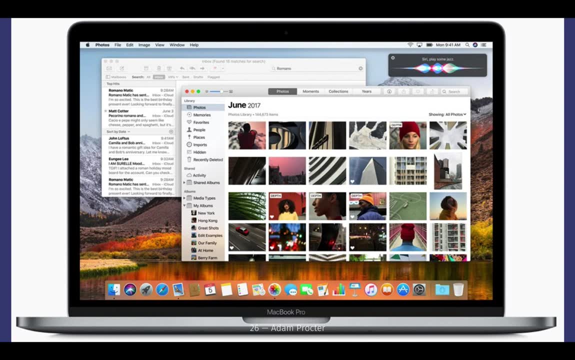 tile metaphor slightly more. but again, most of the operating systems that we undertake that are on computers currently, at least, perform the very, very similar stuff to the system that was created, you know, in 1978, 1979, at xerox park, which is kind of interesting that we've had short history. 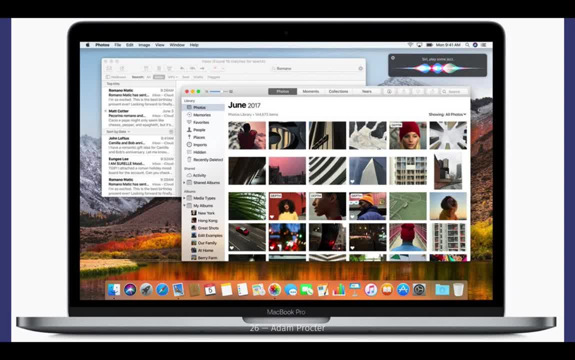 but relatively little change. in fact, the drag and drop files and folder metaphors are very, very similar. so that is a really rapid history of the human computer interaction, particularly focused around where it started and the implementation of the graphical user interface. so a couple of things to reflect upon. 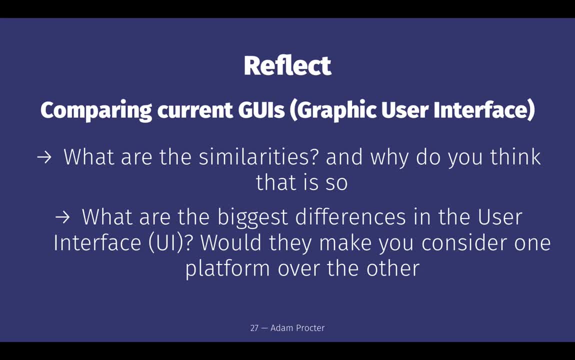 so, comparing current graphical user interfaces, what are the similarities that we see? why do you think that is so? you know, so there's lots of ways that we approach things. why are they similar? and then, maybe, what are the biggest differences in the user interface that you see and would? 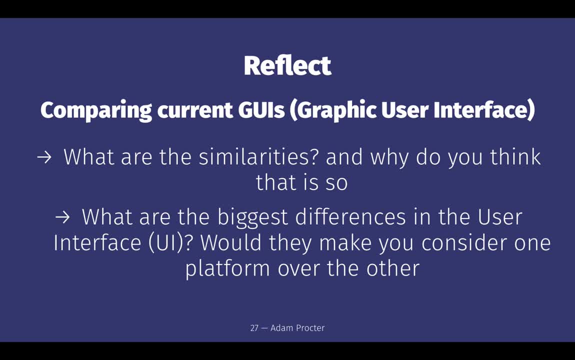 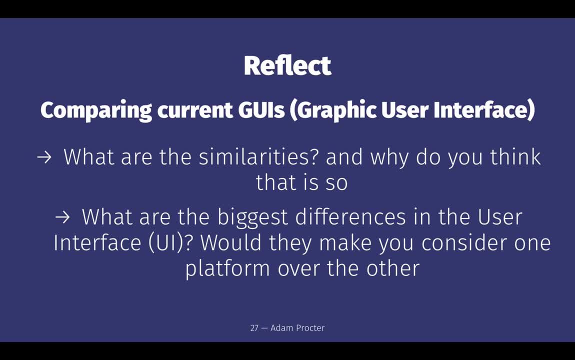 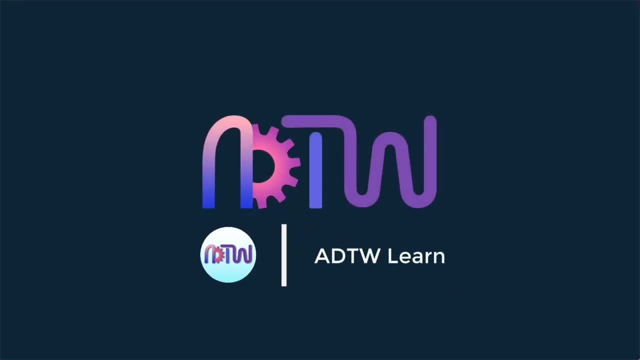 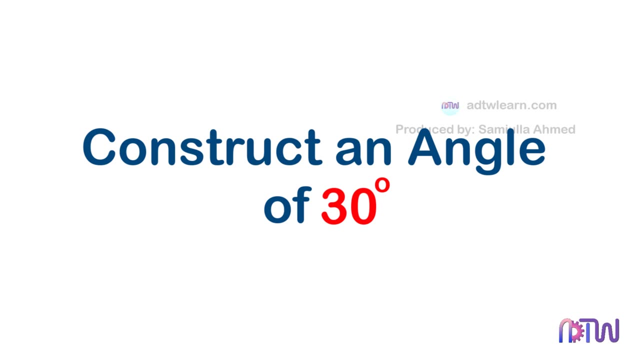 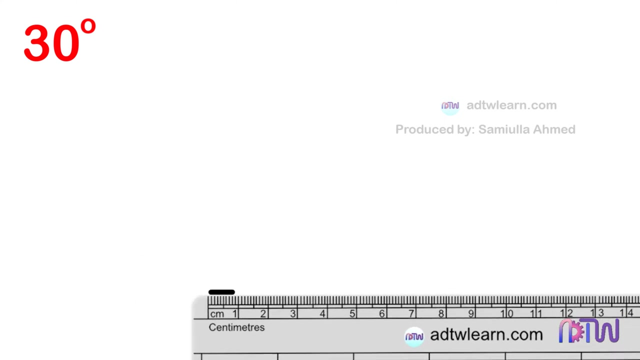 Construct an angle of 30 degree. In this video, we will learn how to construct an angle of 30 degrees using a compass. First, we need to draw a line segment. To do so, take a ruler and draw a line segment and label the endpoints as A and B. Take a compass, adjust it to some length. 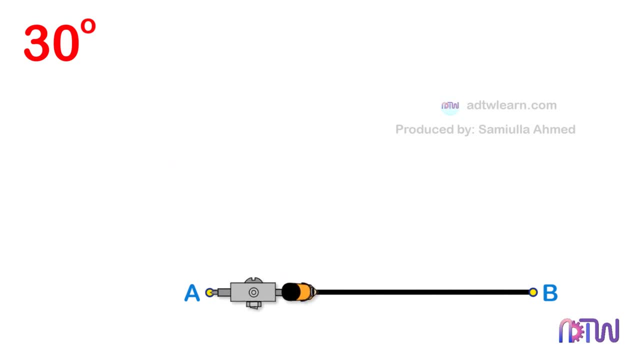 and, using point A as a center, draw an arc as shown. After this, without changing the length of the compass and using this intersection point as a center, cut another arc as shown. Draw a line passing through this intersection point from the endpoint A of the line segment. 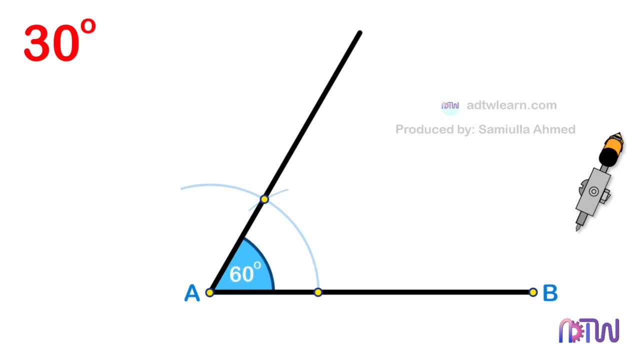 This forms a 60 degree angle. To get the 30 degree angle, we need to divide this angle into half. To do so, take a compass and, using these two intersection points as centers, cut another arc as shown. Finally, draw a line passing through this point from the endpoint A of the line segment. 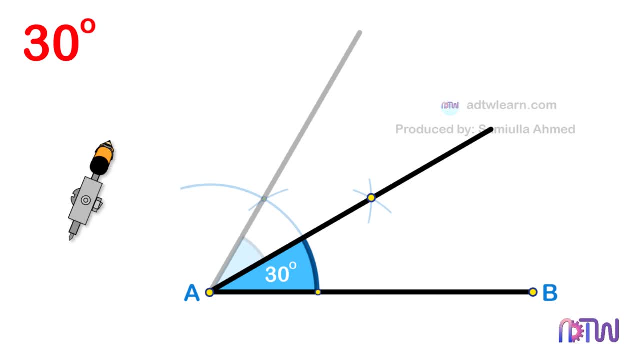 This is the required 30 degree angle. I hope you have understood how to construct an angle of 30 degrees. If you liked this video, please click on the like button and if you are new to my channel, click on the subscribe button and turn on all notifications to get my latest videos.